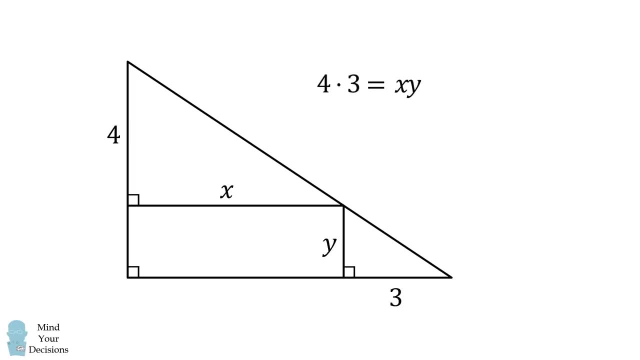 We can then cross, multiply to get that x times y is equal to 4 times 3,, which is equal to 12.. But x times y is exactly the area of the rectangle. Thus the area of the rectangle is always equal to 12.. 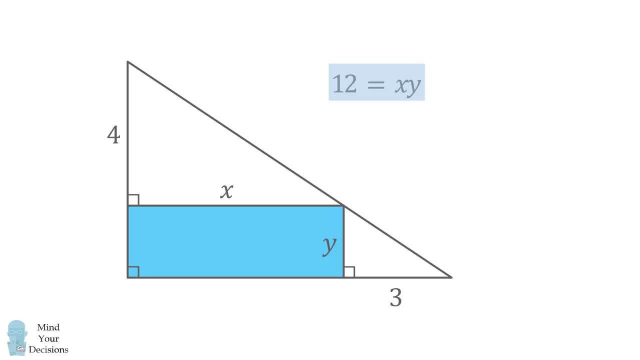 That's the answer to part 1.. Now let's solve for part 2, the minimum area for a triangle that satisfies these conditions. Here is one such triangle that satisfies these conditions. We can measure the base of the triangle and the height of the triangle. 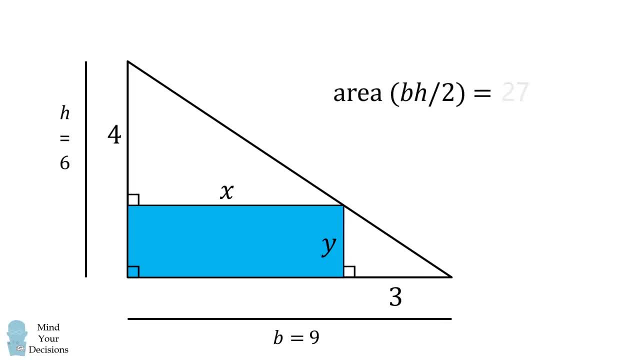 and we'll calculate the triangle's area as 1 half the base times the height. We can then vary the parameters of this triangle. We can change the value of the base of the triangle and the height will adjust accordingly. We'll see that each triangle has a different area. 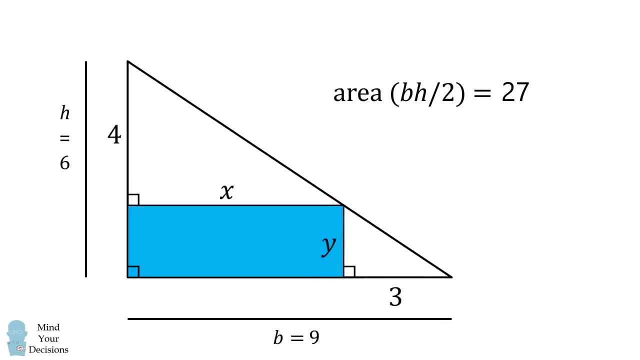 The question is: what is the minimum area for a triangle that satisfies these conditions? How do we solve that? First, we will write an expression for the area of this large triangle. It'll be equal to the sum of the following three areas: 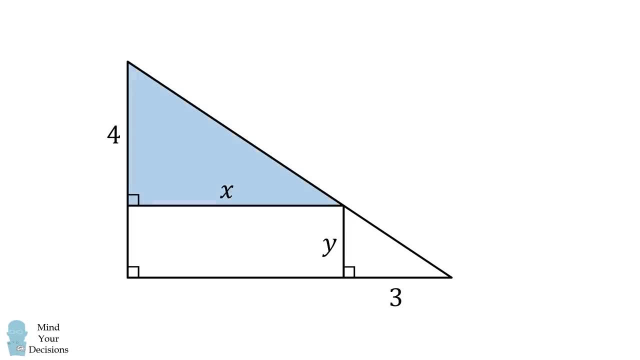 One area is the area of this right triangle. This right triangle has an area that's equal to 4x over 2.. We then add the area of this triangle which is equal to 3y over 2.. Finally, we add the area of this rectangle which is equal to x times y. 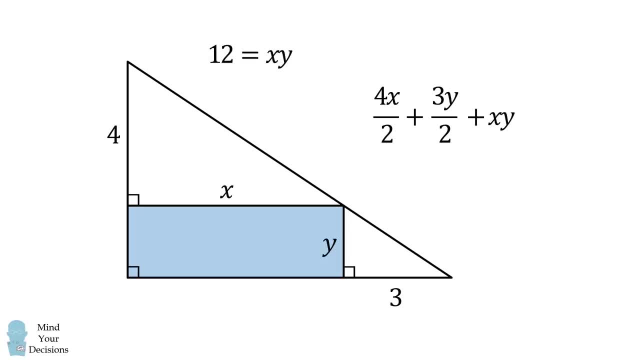 We already solved that x times y is equal to 3y over 2.. So we can substitute that in. Then we can solve this equation for y: y is equal to 12 over x. We can then substitute in for y. We will then simplify this expression. 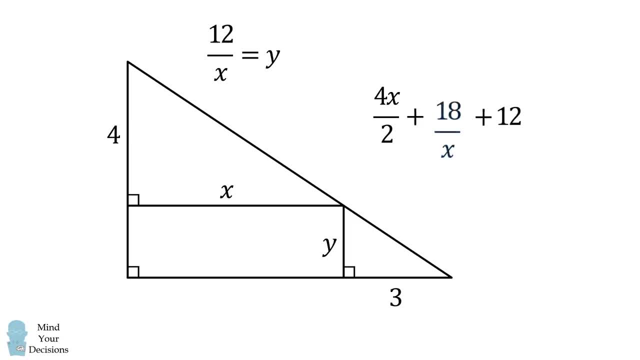 It'll be equal to 18 divided by x. We now have a formula for the area of the large triangle. just in terms of the variable x, It'll be equal to 2x plus 18 over x plus 12.. We'll say: this is f of x and that's the area of the large triangle.